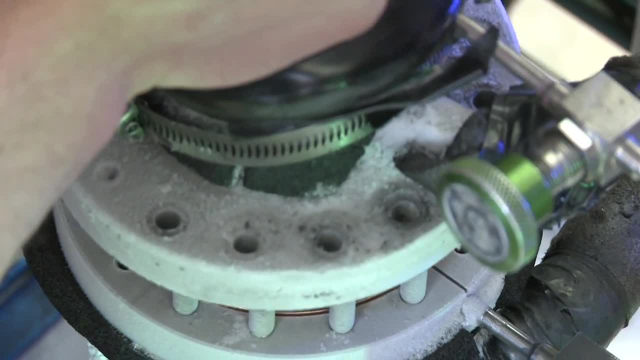 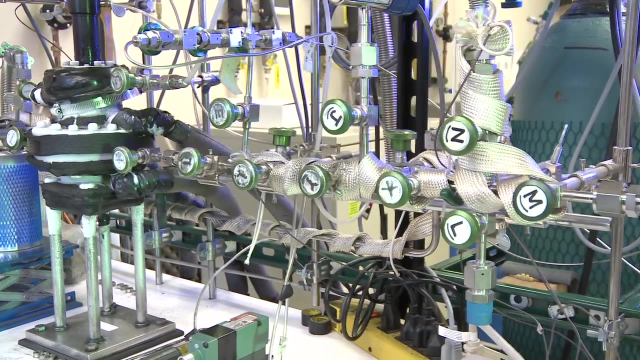 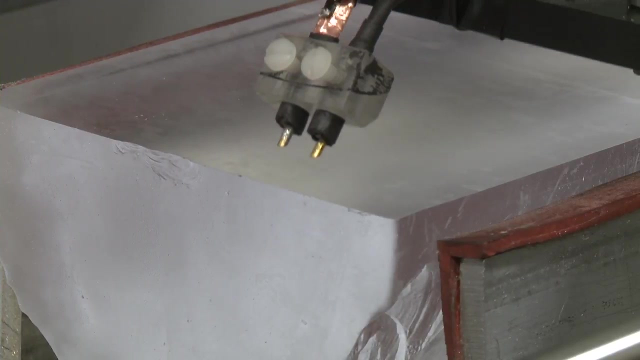 Before crushing the ice, the chamber is tightly sealed and ambient air is pumped out. This isolates the sample of ancient air released. What happens, then is that that air is transported into a gas chromatograph which measures carbon dioxide concentrations. Scientists track the age of a core by 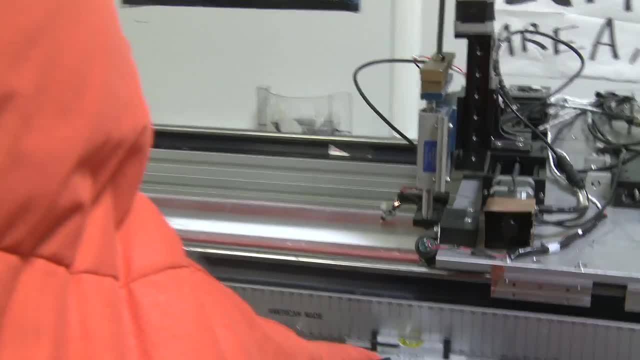 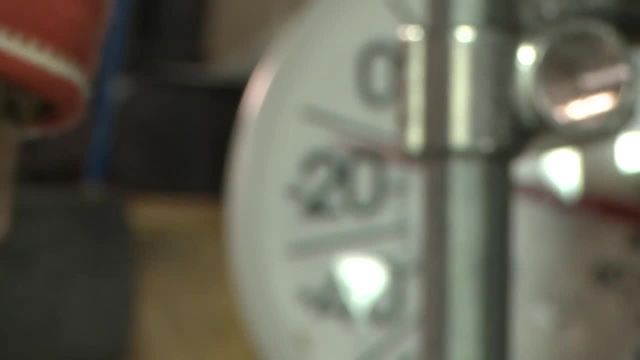 counting its annual layers, which are measured very precisely by changes in electrical conductivity of the ice across summers and winters. The final piece of the puzzle is change in temperature, which can be determined by three different methods. Maybe that you can measure the temperature of the ice by measuring the temperature of the ice. 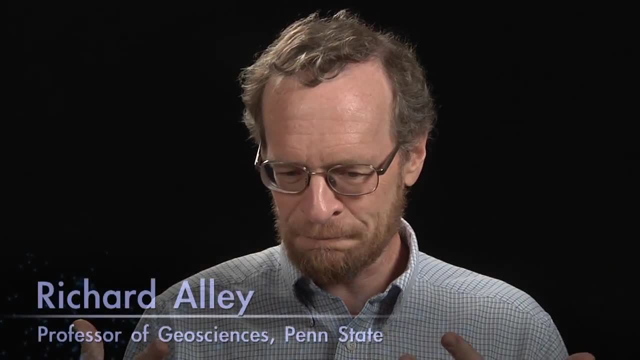 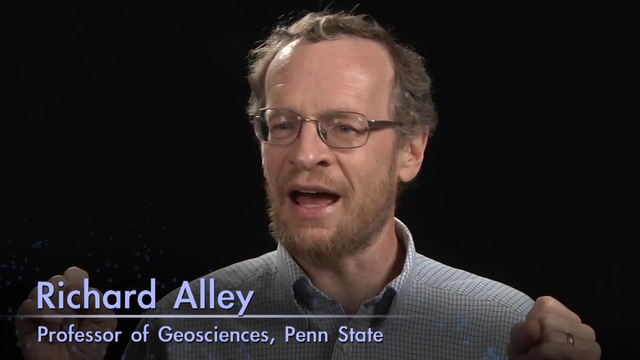 Maybe that you can measure the temperature of the ice by measuring the temperature of the ice. Maybe the easiest one to understand is: if you have a frozen turkey and you put it in the oven and you heat it for an hour, it's still cold in the middle. If you were to drill a hole in your turkey. 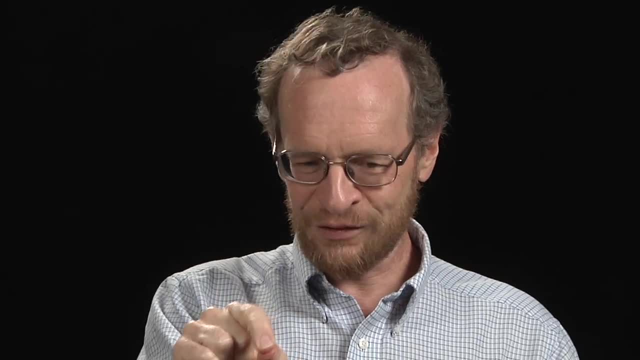 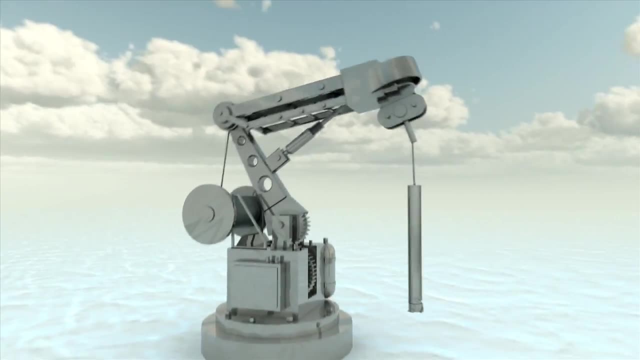 and put a thermometer in, you'd say, wow, it's cold in the middle. This turkey has not been in the oven forever. At one point it must have been in a colder place. You drill a hole in Greenland or in Antarctica and you go down a mile or so. 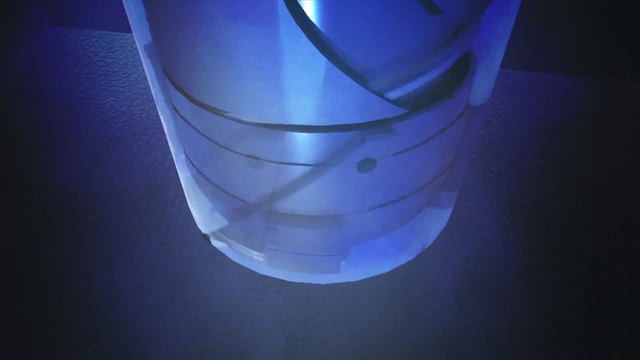 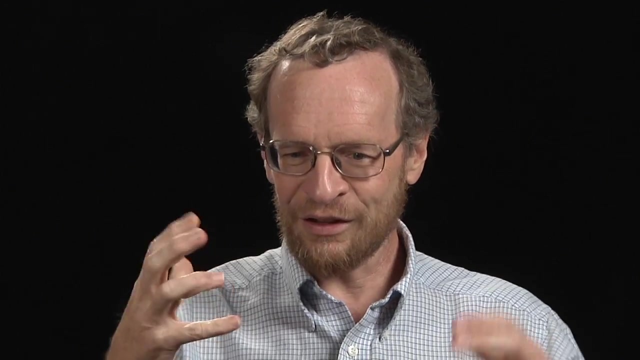 the ice is a little bit colder than it should be, And it's colder than it should be because it hasn't warmed up from the ice age yet. And, in the same way that the turkey was in the freezer, the ice sheet was in the freezer of the ice age And you can learn how cold the ice age was from. 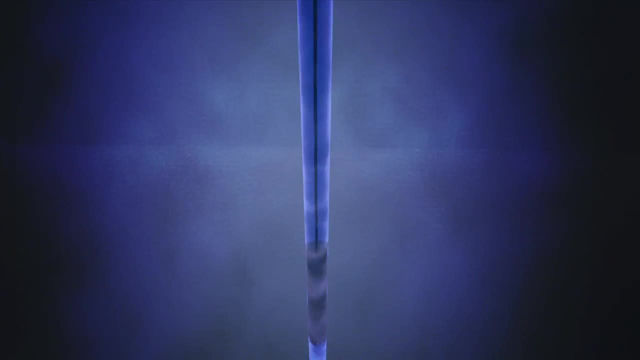 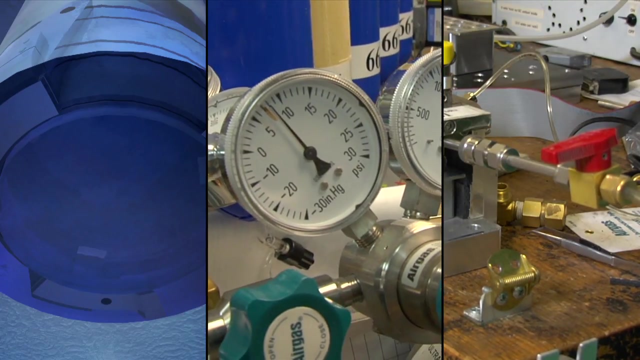 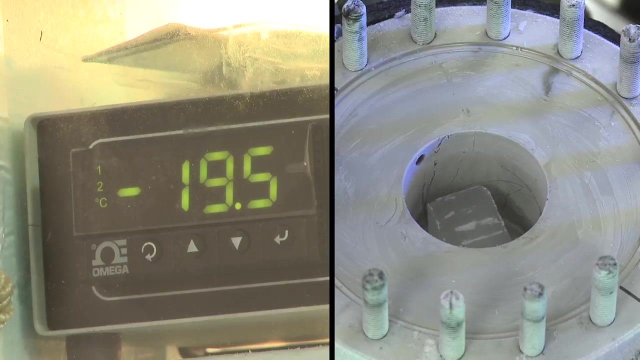 how cold the ice is in the ice sheet. now That's one, There's a couple more as well, And so we start putting together all these different thermometers that you can use, And what we've found so far is they agree with each other By studying how temperature and CO2 concentration 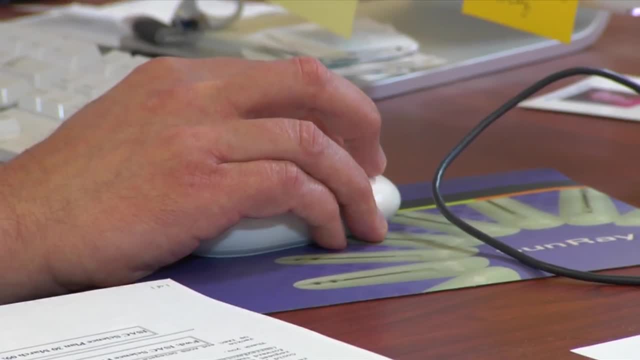 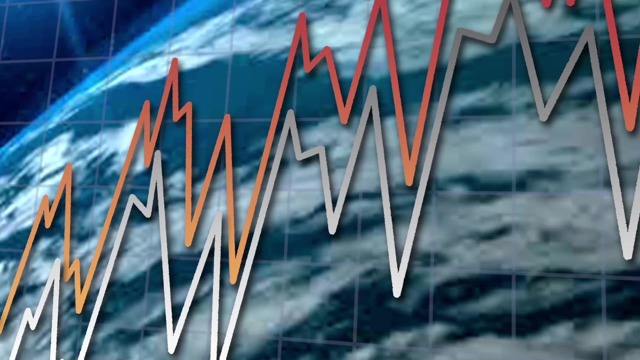 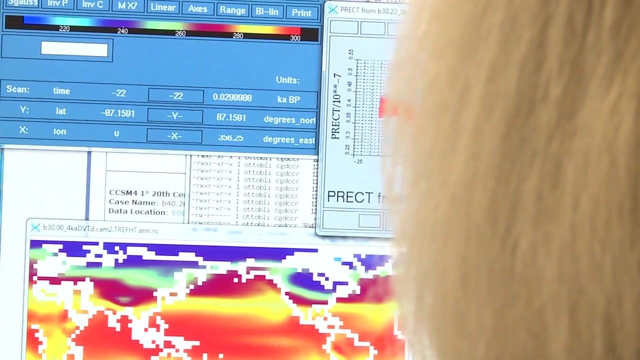 have changed over time. scientists can determine how they are related. Findings show: as CO2 levels increased, so did temperature, And when CO2 decreased, temperatures decreased as well. That information is very useful to climate modelers. Just as climate models can be used to predict the future, they can also simulate the past by 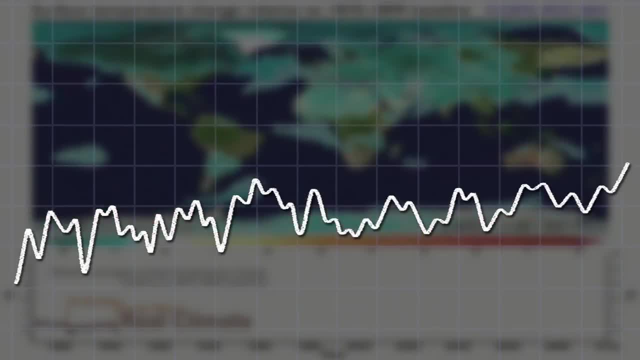 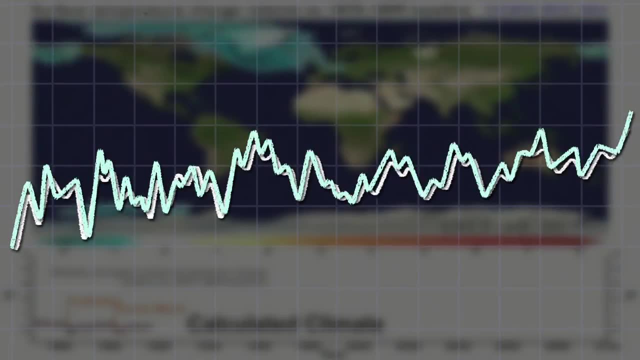 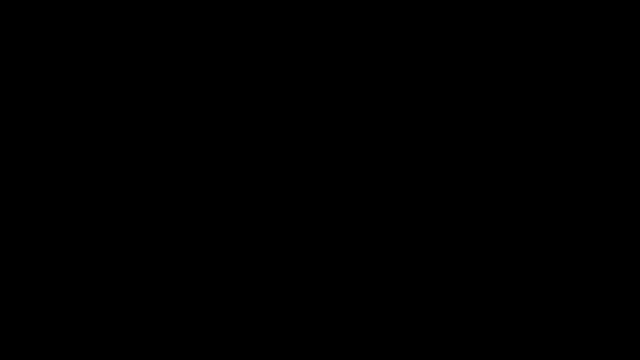 comparing the actual data collected from the ice core record to the numbers calculated by computer models, Researchers have shown these models to be highly accurate. This gives scientists the confidence to employ those same models for the prediction of future conditions. But why does our climate change? What are the factors that influence its variability? 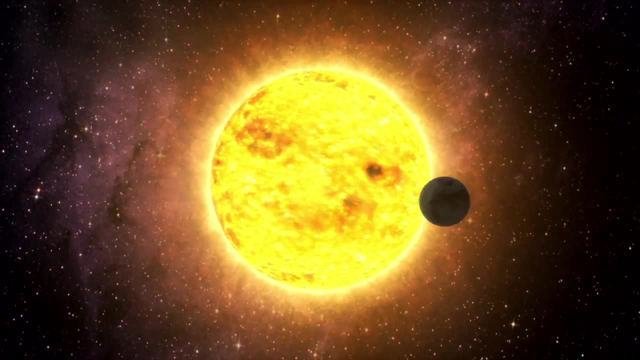 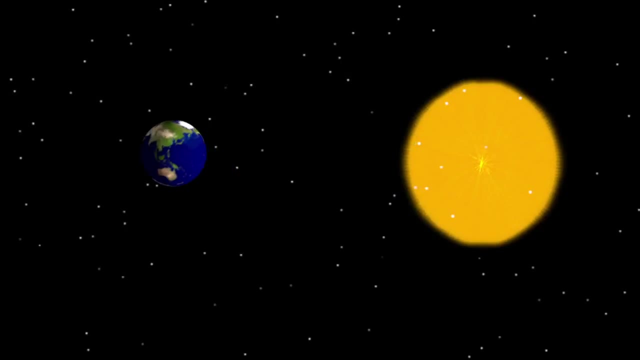 The amount of energy we get from the sun changes. I think we can understand that very simply when we look at summers and winters. When we're in a summer, we're tilted towards the sun and we get more sun's energy in the northern hemisphere, In the southern hemisphere. 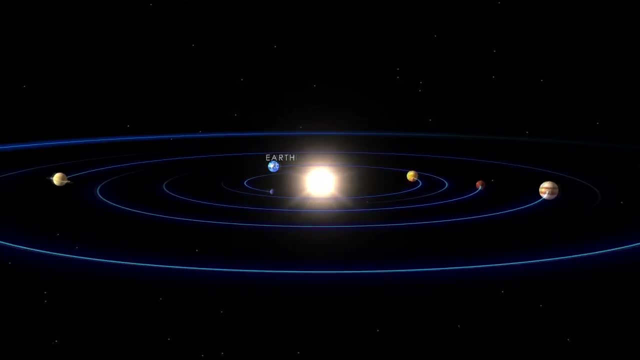 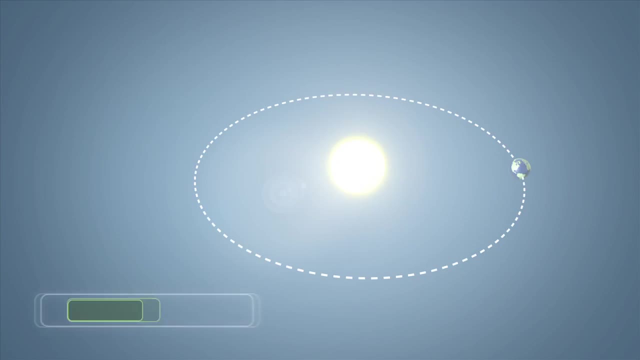 it's winter because they're tilted away from the sun. We get the same kind of thing happening over thousands of years as the earth's orbit changes. So imagine at a time we are farther away from the sun, we get less solar energy, And there 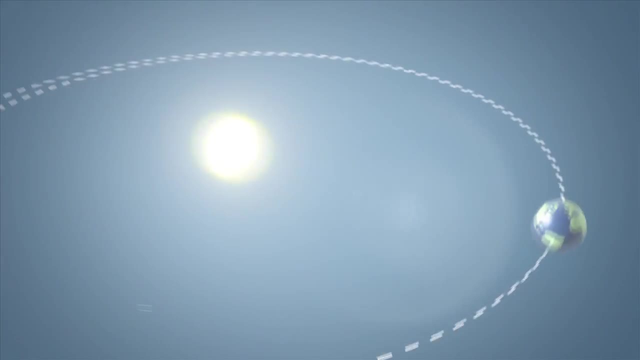 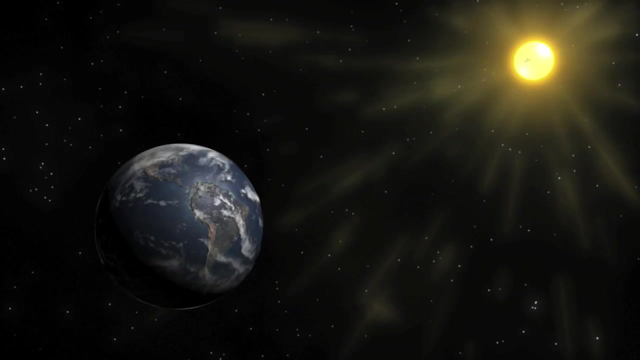 are times when we're closer to the sun, we get more solar energy. When we're closer to the sun, we have a warmer planet. When we're farther away from the sun, we have a colder planet. It turns that when the earth is warmer, when we're closer to the sun, we also have higher levels of CO2. 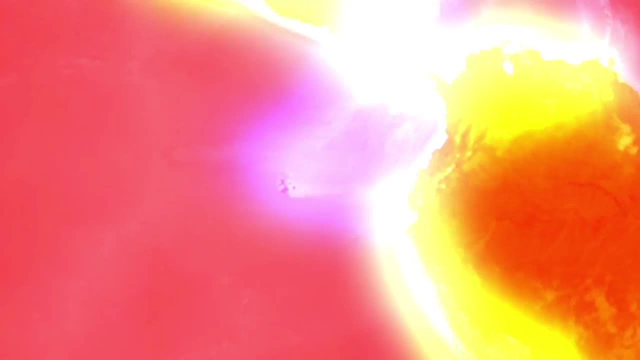 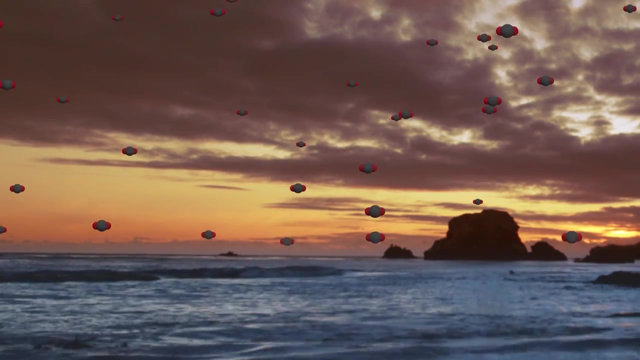 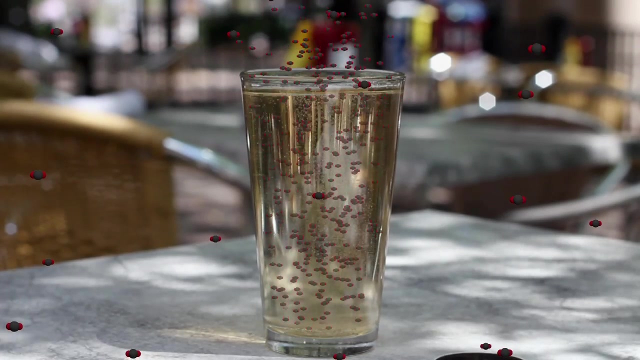 in the atmosphere. Why is it that when we have a warmer planet, we get more CO2 in the atmosphere? One reason is that as the planet warms, the ocean's ability to absorb CO2 decreases. Imagine a recently opened can of soda. Over time, carbon dioxide moves from the soda water into the 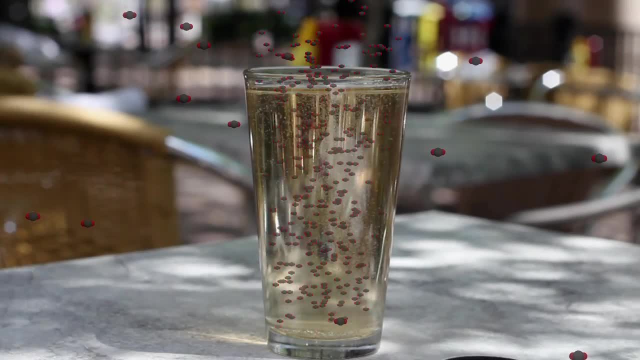 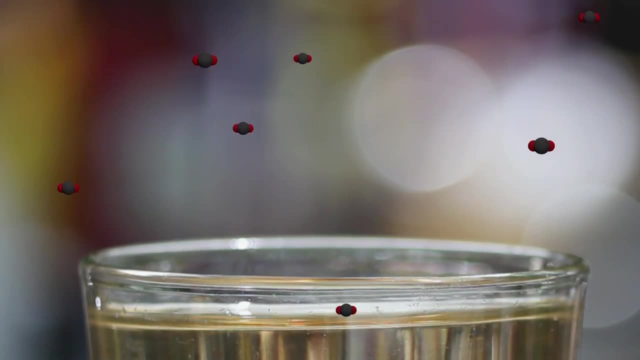 air, leaving the soda flat. This happens because there is a higher concentration of CO2 in the soda relative to the surrounding air. However, if there were a higher concentration of CO2 in the air, carbon dioxide would move in the opposite direction- into the soda. 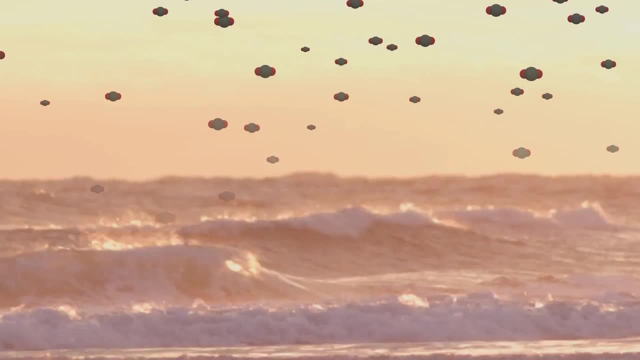 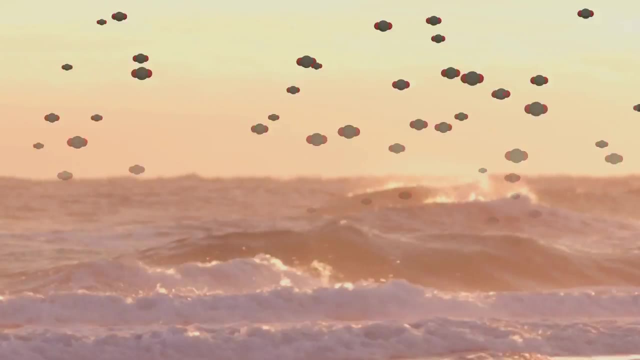 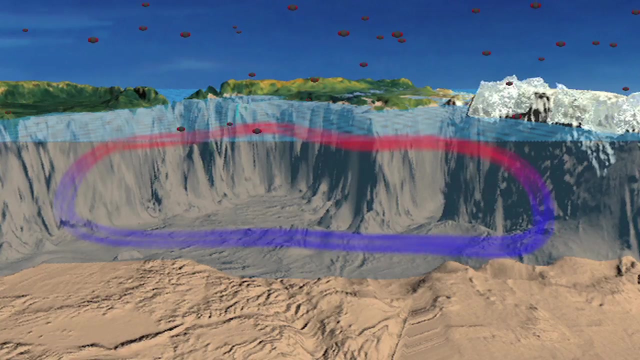 Apply that same principle to the ocean, Because there is more CO2 in the atmosphere than at the surface of the ocean, carbon dioxide mixes into the water, But as the planet warms, ocean currents change, altering the exchange of CO2 between the air and the water. 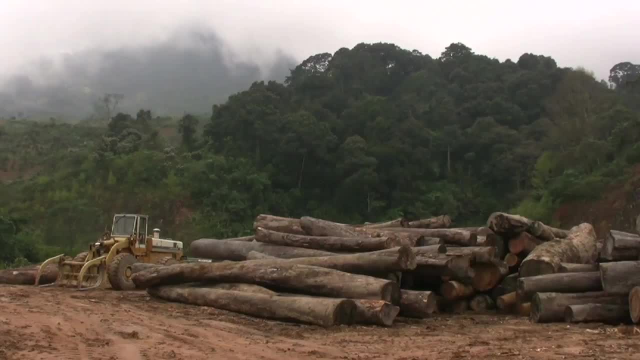 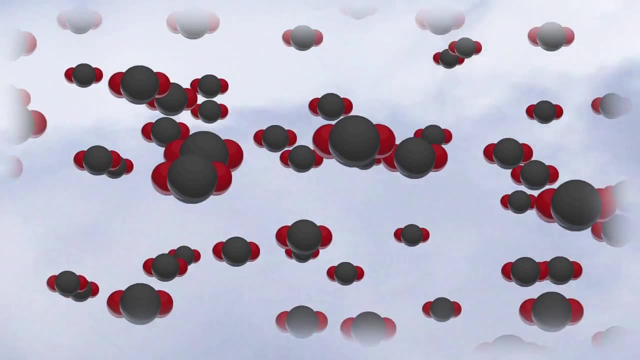 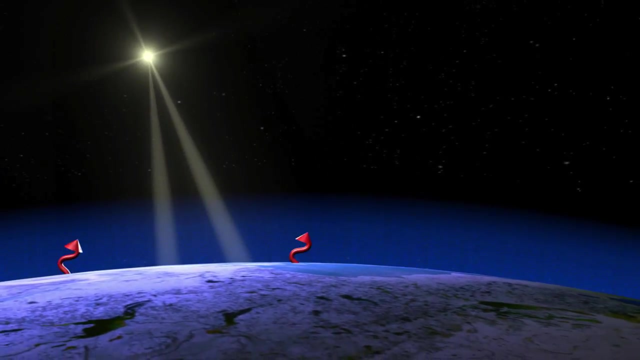 Changes in the amount of sea ice and the biosphere also influence the amount of CO2 in the air. An increased concentration of carbon dioxide makes the planet even hotter, And that is due to the greenhouse effect. In a greenhouse, we want to keep the air warmer than it is in the outside world.